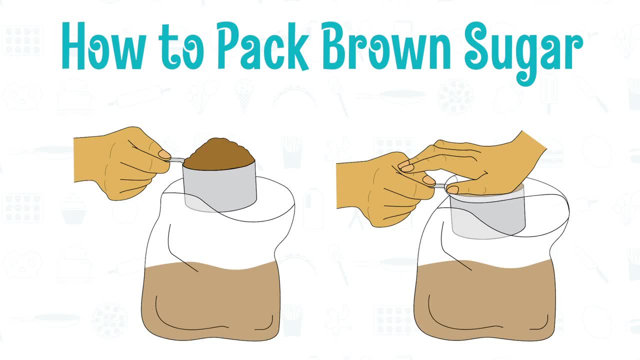 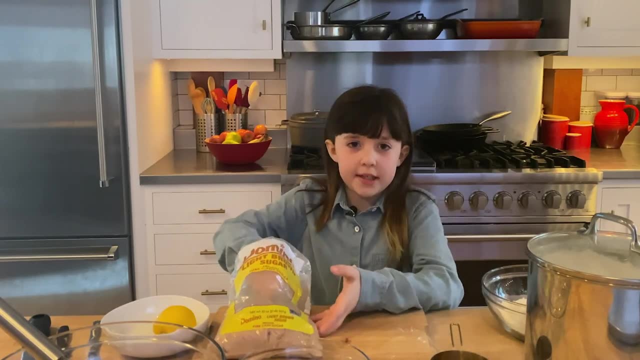 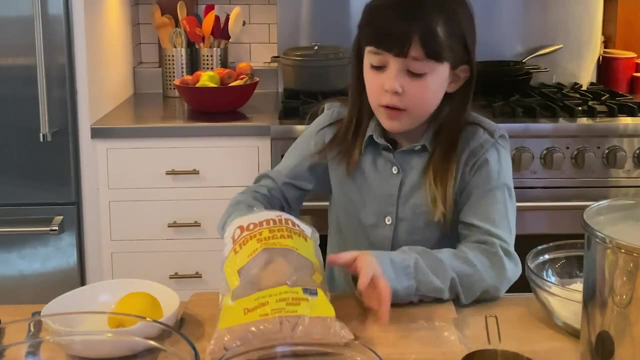 in the bowl. So now we're going to teach you how to pack brown sugar. It's the opposite of flour, because you want to make sure you pack it. You can usually scoop it and then leave it in the bag, and then you want to press the top of the bag If you don't. 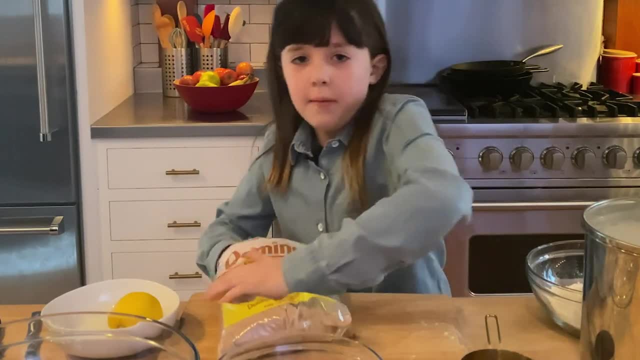 have enough, then you can just add more and then press it again, and then you want to tap it, And it's okay. if you don't have enough, you can just add more and then press it again, and then you want to tap it, and it's okay. 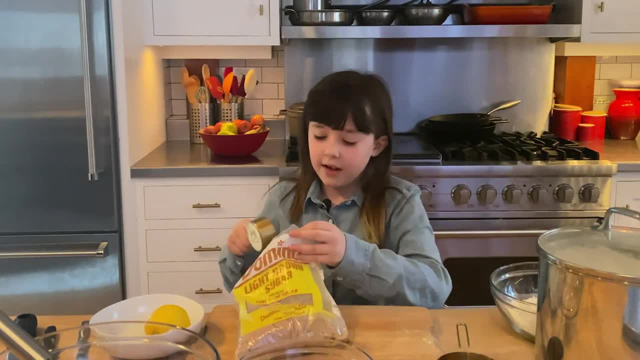 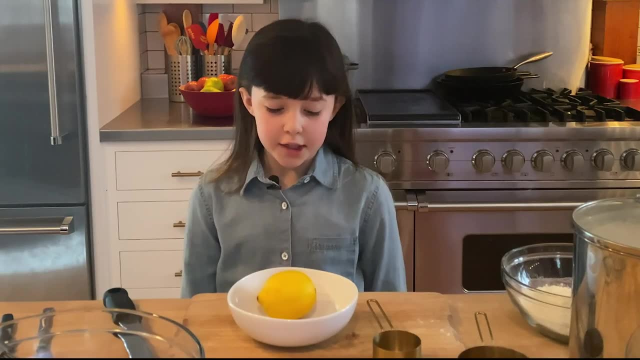 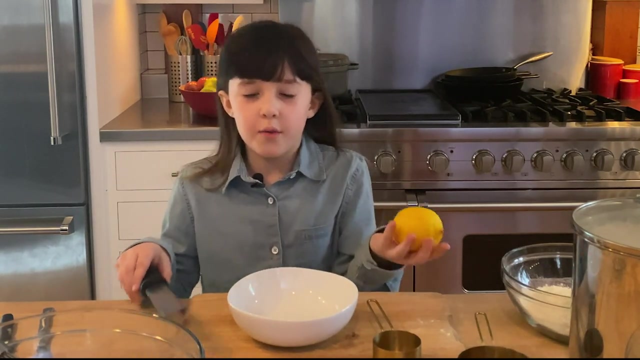 If it's stuck together, it's usually because you press it, so it's packed Next up. I'm going to teach you how to zest a lemon. You want to be really careful that you don't just hold the lemon normally like you're getting it out of the fridge. You want to make sure that. 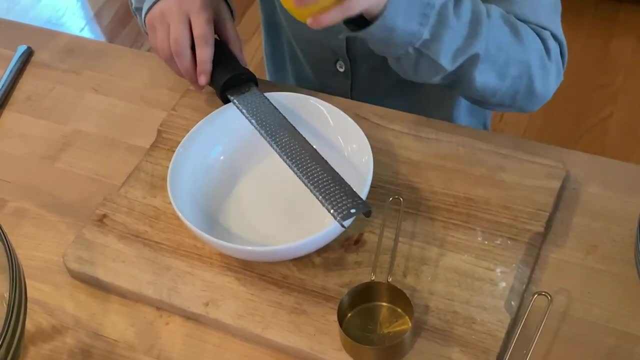 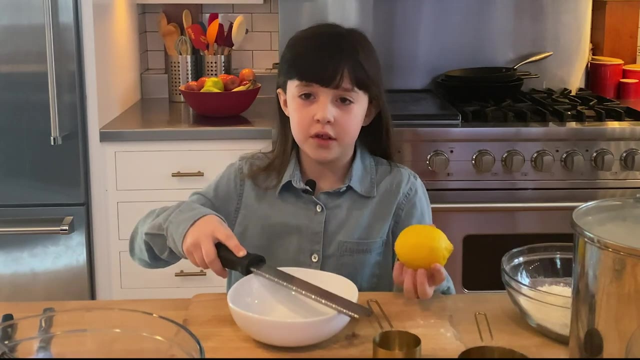 you use a claw because if you're just holding it, you can scrape yourself. I use a claw and I'm also using a Microplane. If you don't have this, you can use a just a normal zester. So you want to make a clot? 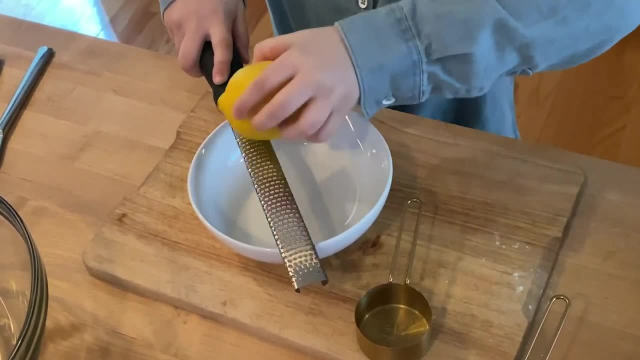 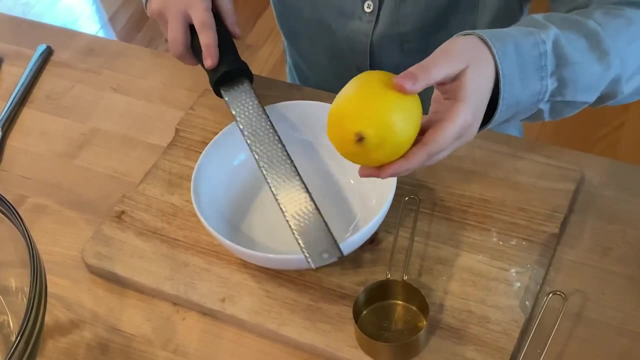 and then you want to just move it back and forth and make sure. you want to make sure you're moving the lemon or the fruit you're zesting, not this, because then the fruit just goes with it and it can also scrape whatever you're using. 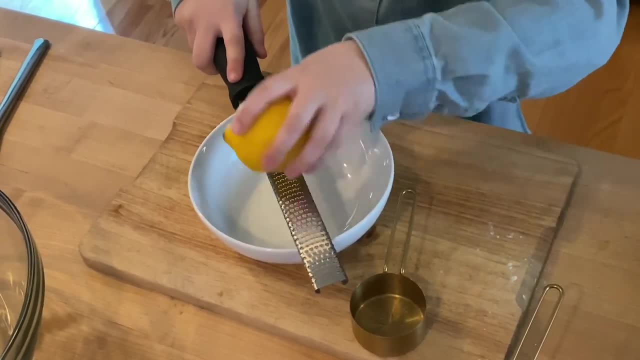 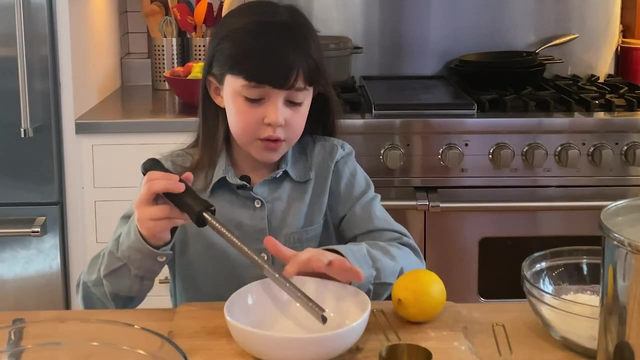 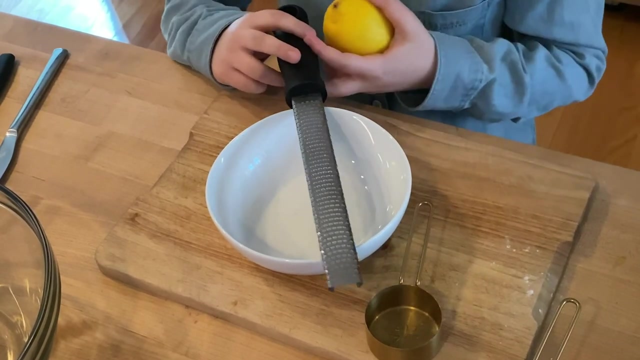 to get the thing you zest into the bowl And then, once you've done that, there might be a little some zest in the thing. So you just want to make sure that you get all of it out, And if there's nothing, then you can just leave. 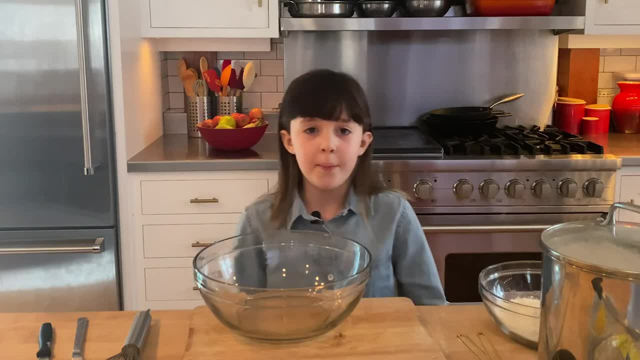 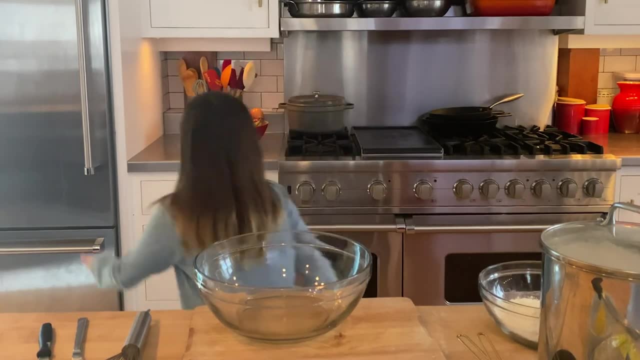 The last thing I'm gonna show you is to make whipped cream. First, you want to make sure that your cream is very cold. You want to get it right out of the fridge, because if it's warm it can be hard to whip. 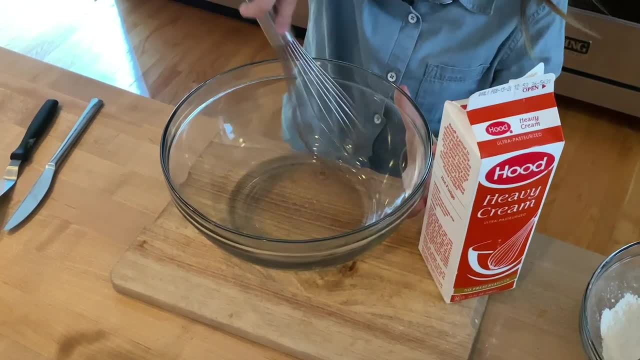 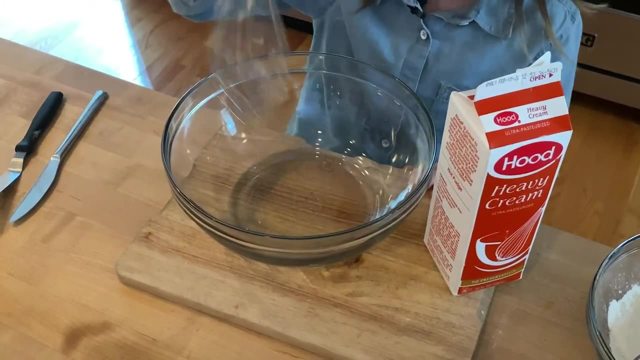 And you want to make sure that you're not just going like this. You want to make sure that you're really beating it. So because if you're just going like this, that's going to take a while and it's going to waste a lot of time.